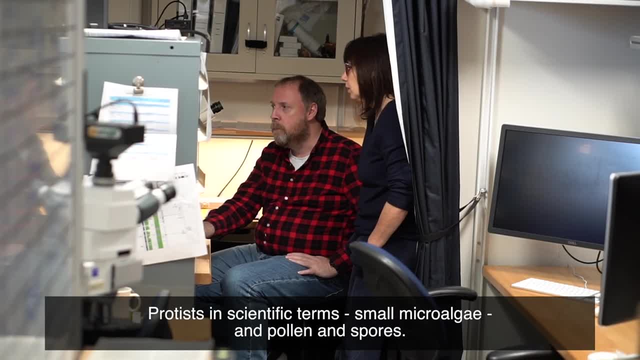 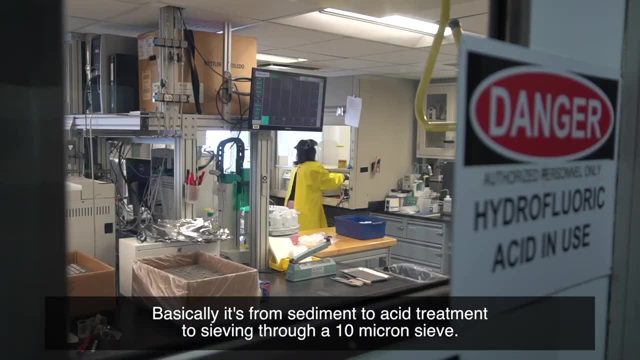 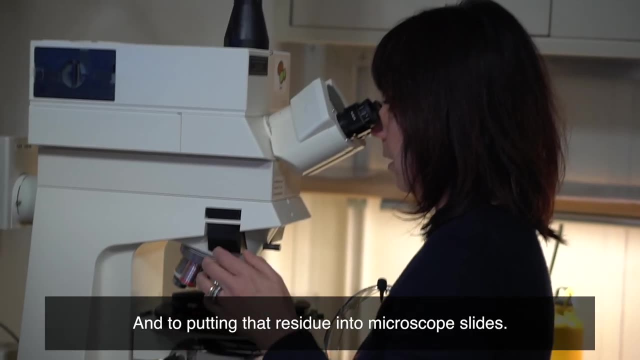 you can think about, and pollen spores, so remains or fossils of ancient or present vegetation. So basically it's from sediment to acid treatment, to sieving through 10 micron sieves and to putting that residue into microscope slides, and then I can go to the microscope and look. 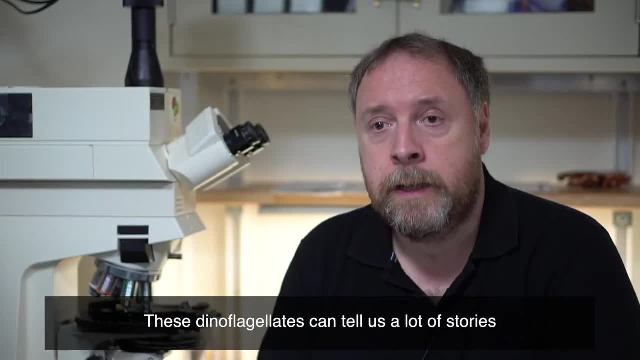 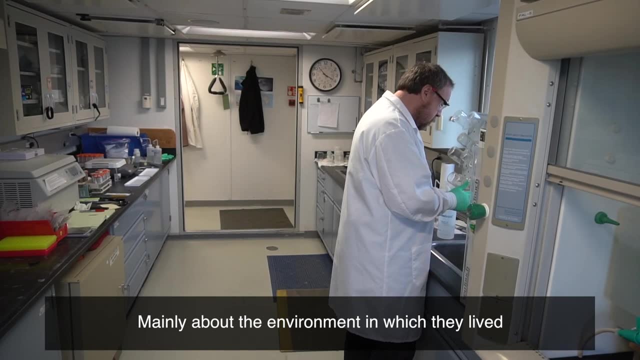 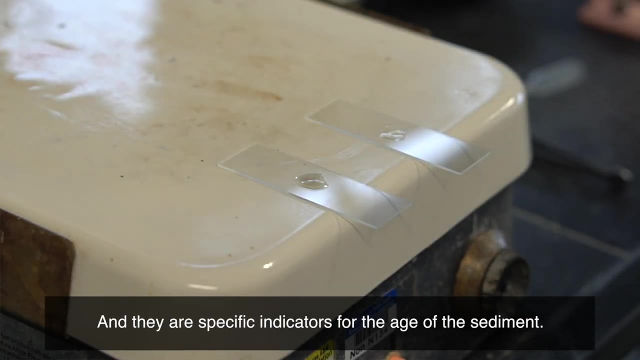 at the fossil that I've found. These dinoflagellates can tell us a lot of stories, mainly about the environment in which they lived before they died, And thank to the… Oh …seafloor, and they are specific indicators for the age of the sediment. 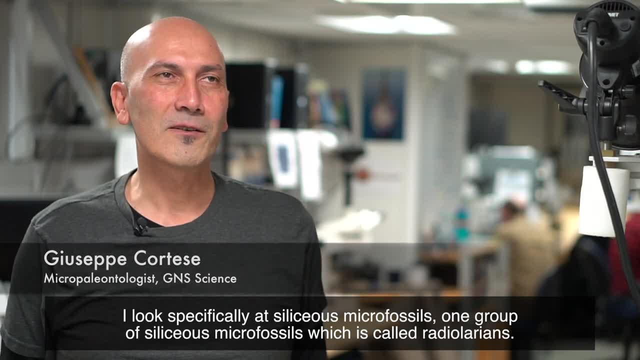 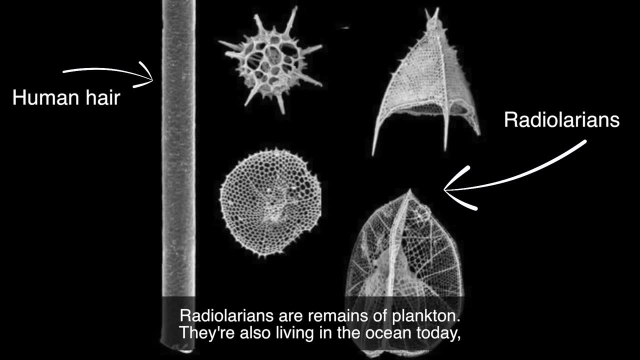 I look specifically at siliceous microfossils, one group of siliceous microfossils which is called radiolarians. Radiolarians are remains of plankton. they're also living in the ocean today, but I look at their fossilized remains. 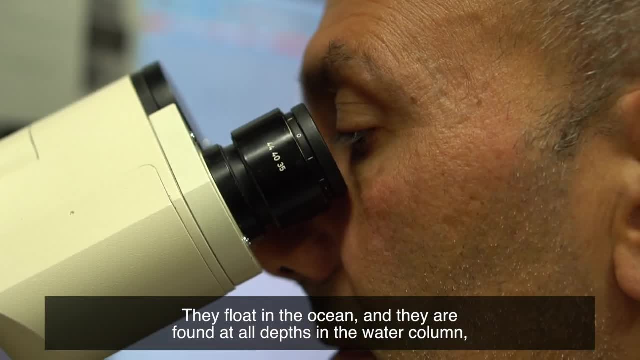 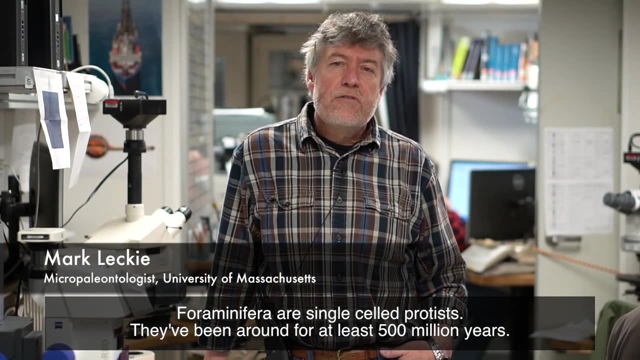 They float in the ocean and they are found at all depths in the water column, from the very surface down to… …thousands of meters of depth. Forminifera are single-celled protists. They've been around for at least 500 million years. 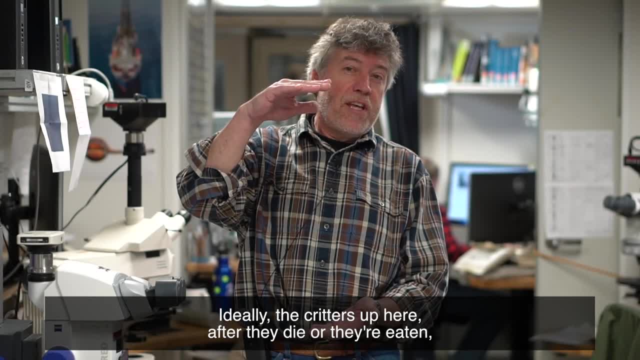 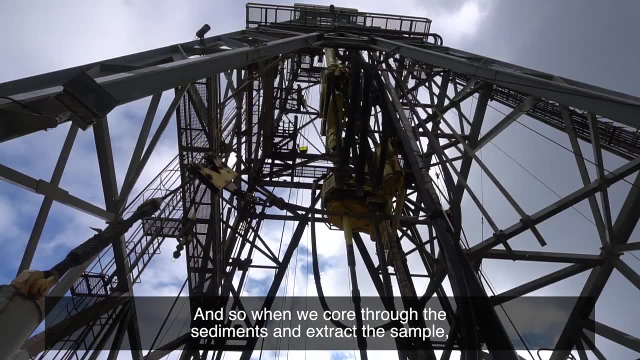 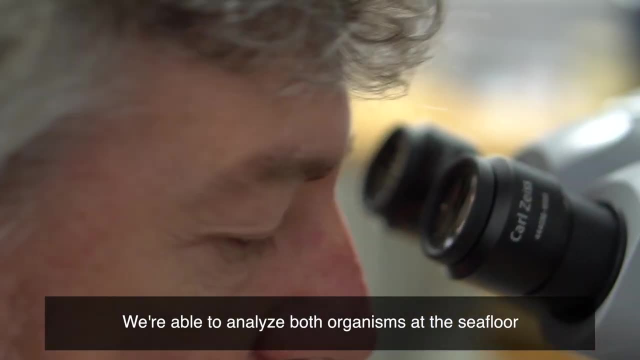 Ideally the critters up here. after they die or they're eaten, they accumulate on the seafloor with the sediments, And so when we core through the sediments and extract the sample, we're able to analyze both organisms at the seafloor and the ones at the surface. 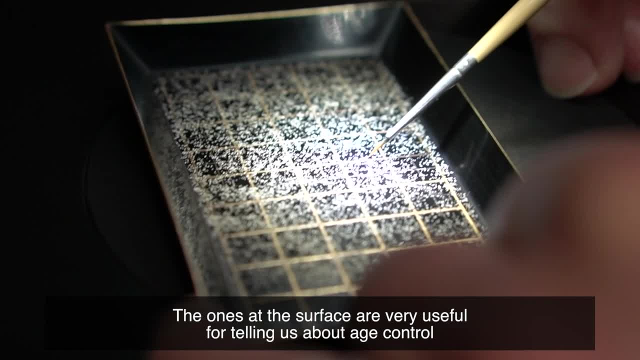 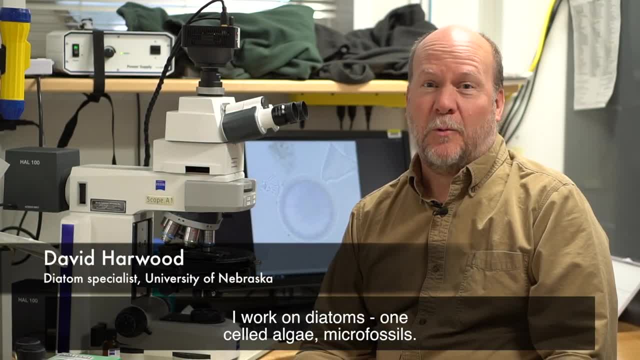 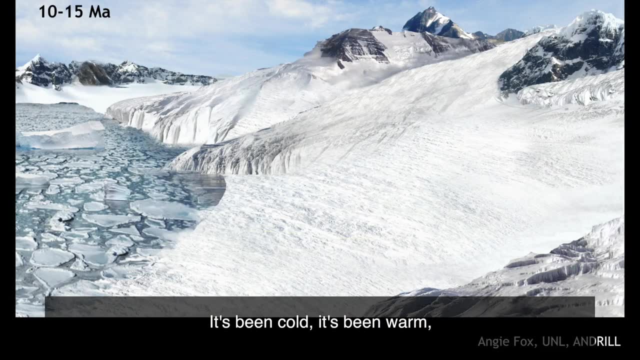 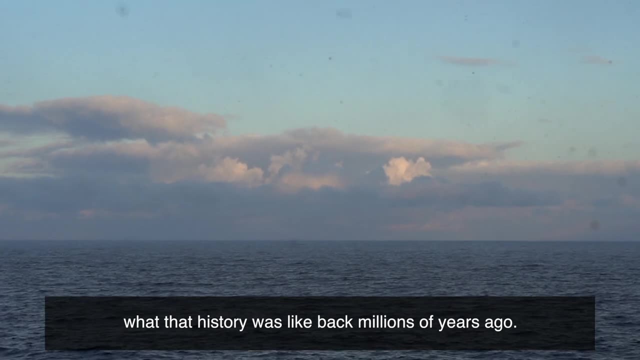 environment. I work on diatoms, one-celled algae, microfossils, and Antarctica's changed a lot through time. It's been cold, it's been warm, and the microfossils we study are one of the clues that we use to try to figure out what that history was like back millions of years ago. 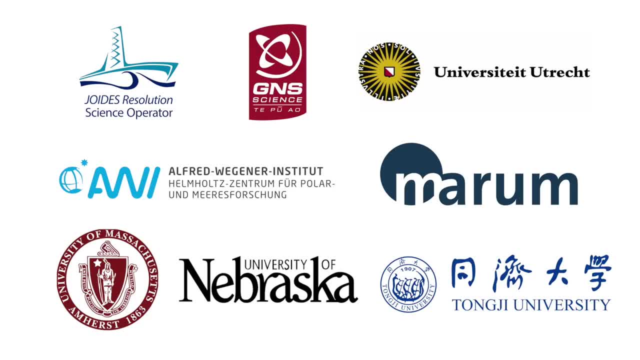 I've got to admit, I've tried to learn how to use them and I really mean to…. But even if you were doing a science project and you're thinking, well, it's not going to change anything, it's going to… …it's going to stop. It's going to stop, It's going to start. I'm taking that away from you. Okay, I… …I'm taking that away. I'm taking that away from you.